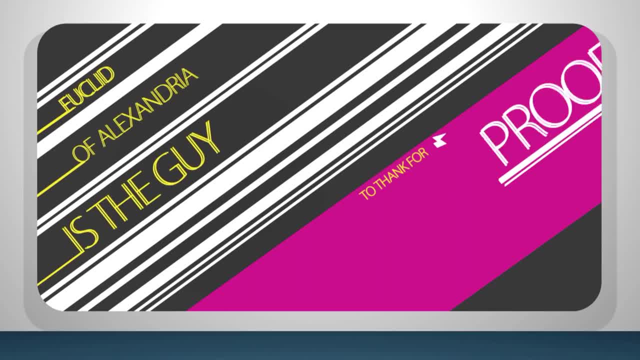 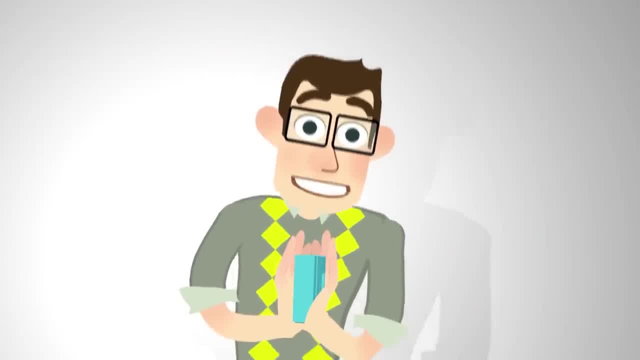 fan mail. Euclid of Alexandria is the guy to thank for proofs. Euclid is not really known for inventing or discovering a lot of mathematics, but he revolutionized the way in which it is written, presented and thought about. Euclid set out. 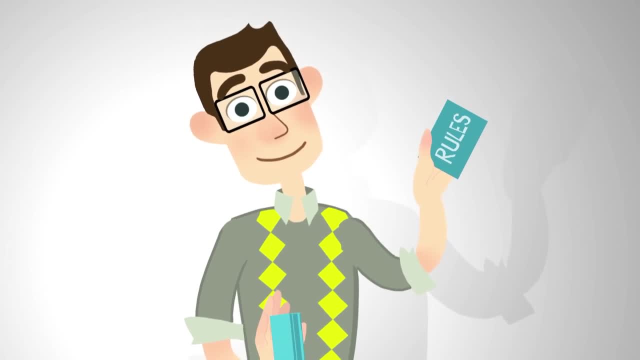 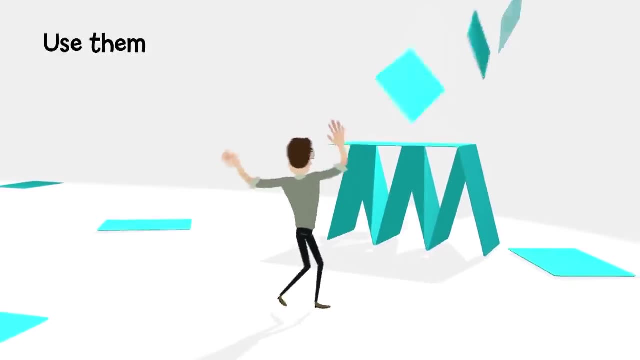 to formalize mathematics by establishing the rules of the game. These rules of the game are called axioms. Once you have the rules, Euclid says, you have to use them to prove what you think is true. If you can't, then your theorem or idea might be false. And if 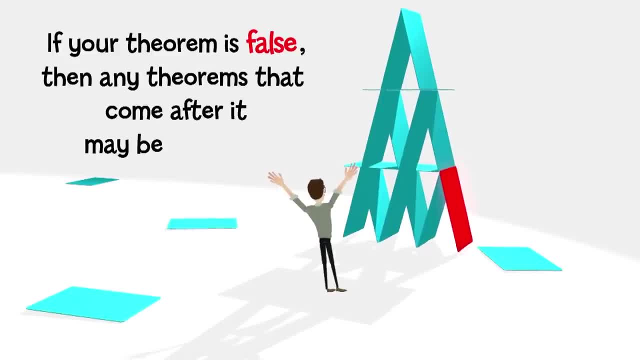 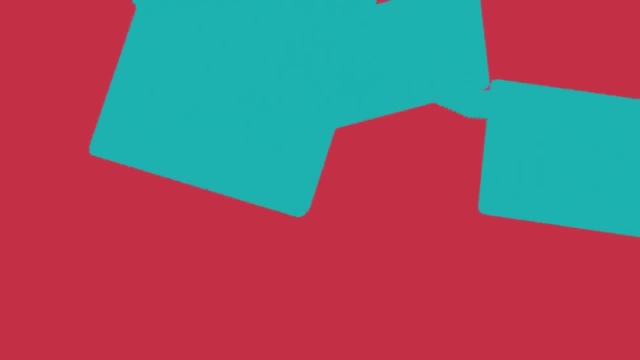 your theorem is false, then any theorems that come after them are false. it and use it might be false too, Like how one misplaced beam can bring down the whole house. So that's all. the proofs are using well-established rules to prove beyond a doubt that some theorem 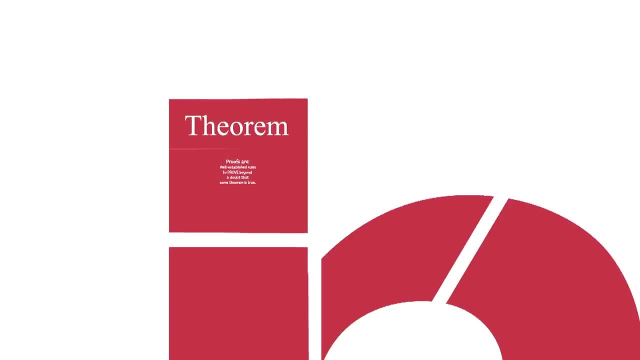 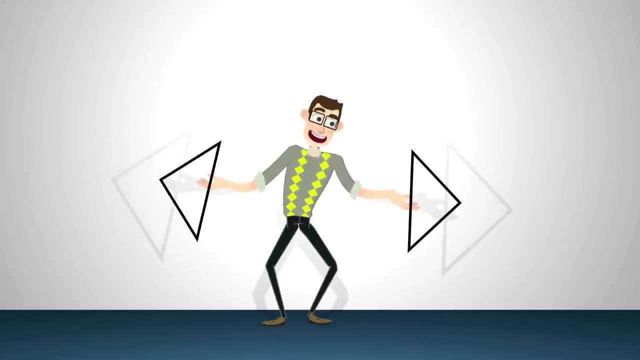 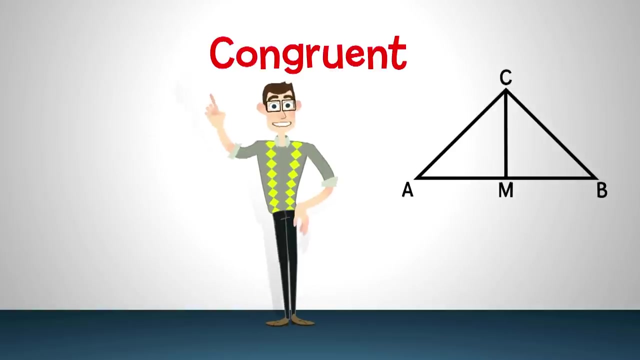 is true, Then you use those theorems like blocks to build mathematics. Let's check out an example. Say, I want to prove that these two triangles are the same size and shape, In other words, they are congruent. Well, one way to do that is to write a proof that shows that all three sides of one triangle 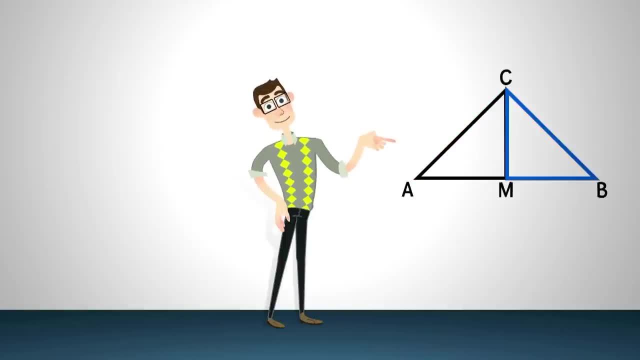 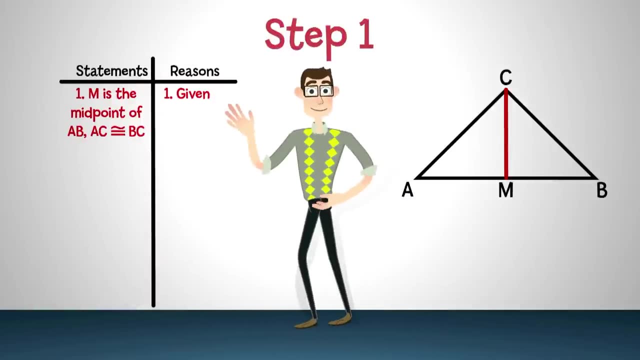 are congruent to all three sides of the other triangle. So how do we prove it? First I'll write down what we know. We know that point M is the midpoint of AB. We also know that sides AC and BC are already congruent. 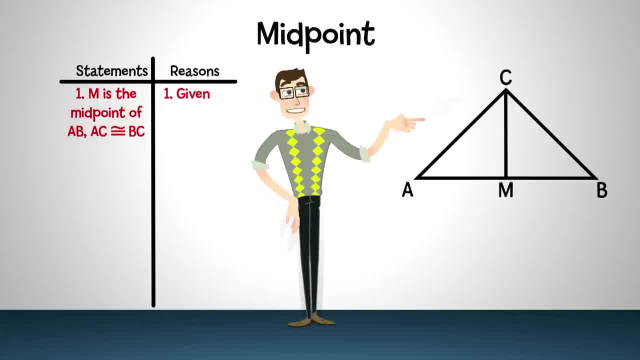 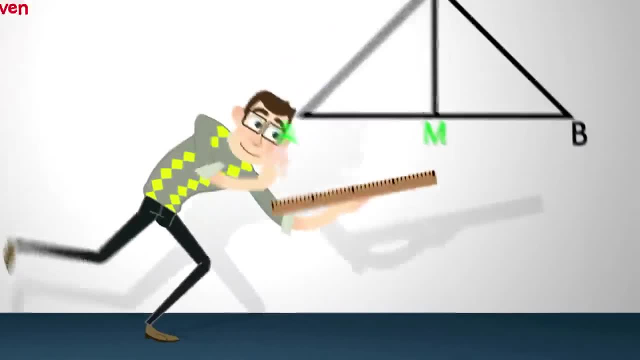 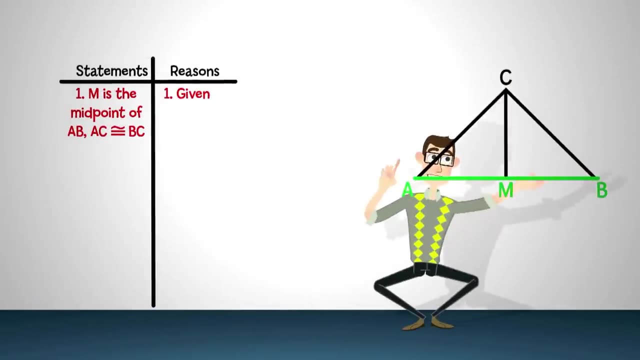 Now let's see what does the midpoint tell us? Luckily, I know the definition of midpoint: It is basically the point in the middle. What this means is that AM and BM are the same length, since M is the exact middle of AB, In other words, the bottom side of each of our triangles- are congruent. 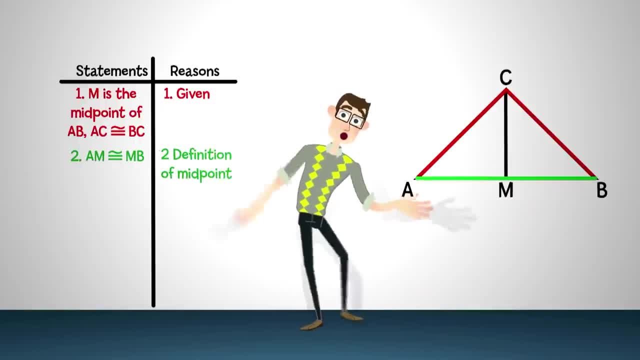 I'll put that as step 2.. Great, So far I have two pairs of sides that are congruent. The last one is easy: The third side of the left triangle is CM And the third side of the right triangle is well, also CM. 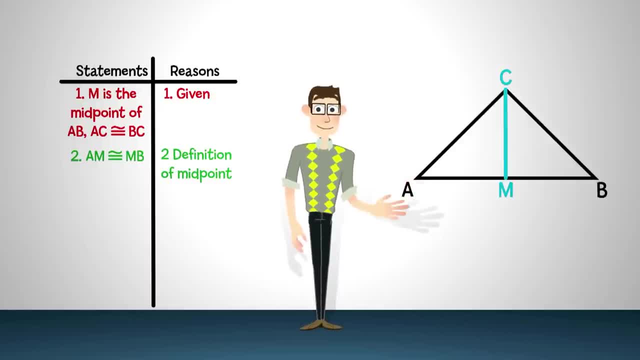 They share the same side. Of course it's congruent to itself. This is called the reflexive property. Everything is congruent to itself. I'll put this as step 3.. Ta-da, You've just proven that all three sides of the left triangle are congruent to all three.